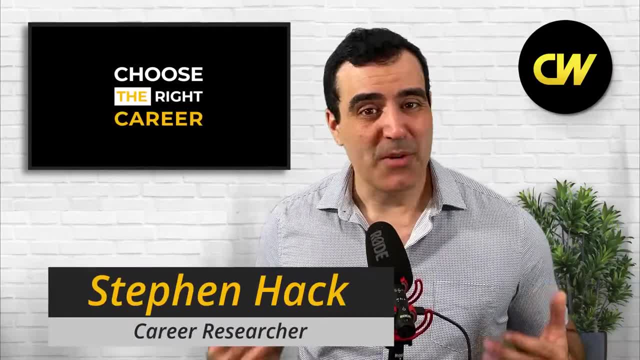 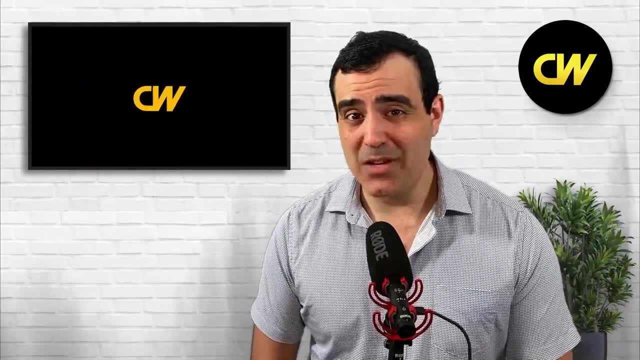 Should you become an environmental engineer in 2022?? The purpose of this video is to help you figure out whether this career is for you. We're going to go over different facts and figures, including salaries, demand, work environment, demographics and more Environmental engineers. 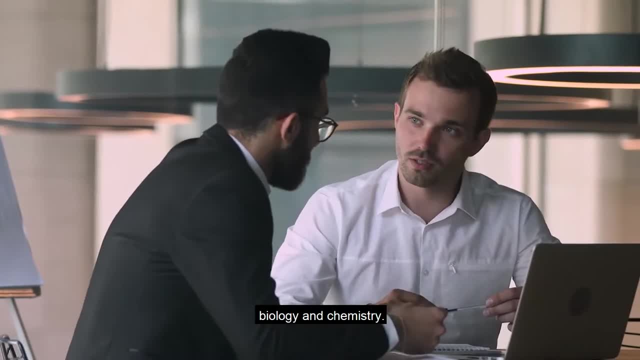 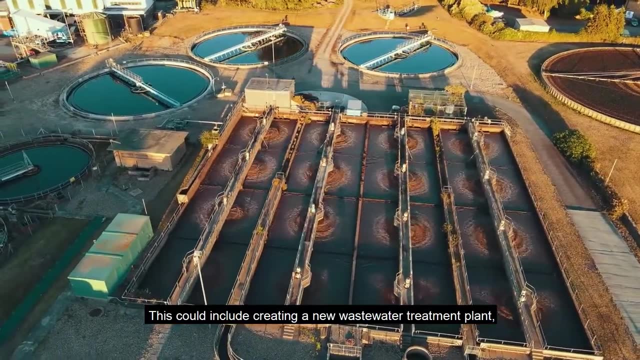 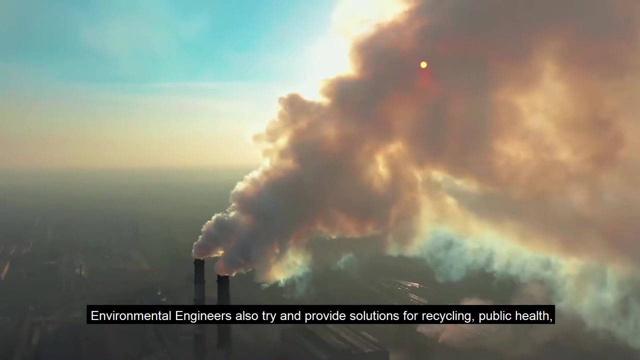 are experts in engineering, social science, biology and chemistry. They develop modern-day solutions to environmental problems. This could include creating a new wastewater treatment plant, site remediation, pollution control technology and dealing with hazardous waste. Environmental engineers also try and provide solutions for recycling, public health and air pollution. 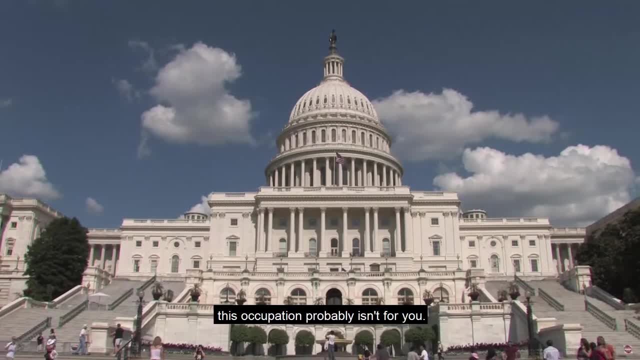 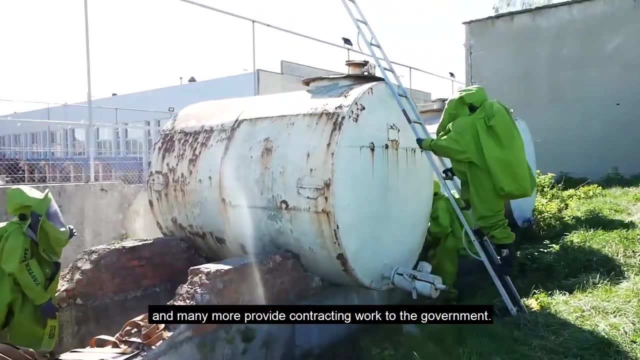 If you don't like working with the government or for the government, this occupation probably isn't for you. 26% of environmental engineers work for a state, local or federal government, and many more provide contracting work to the government. Often, environmental engineers are: 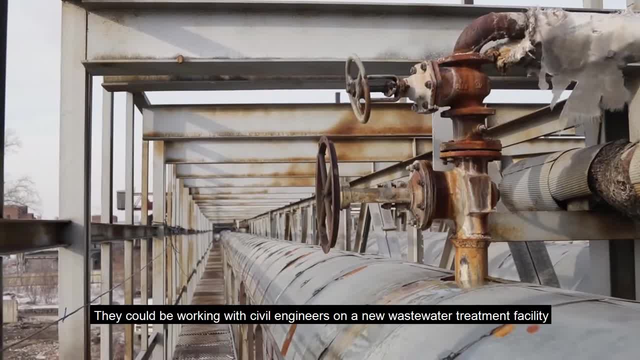 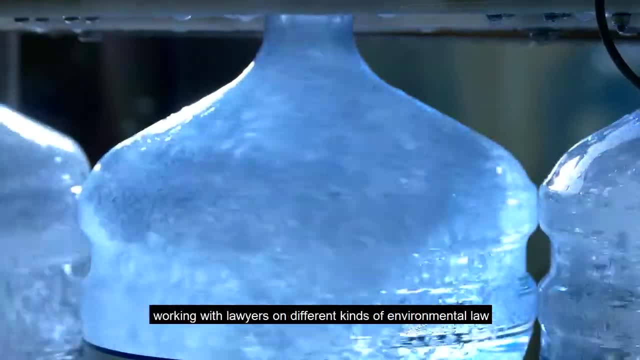 working with other professionals to achieve their goals. They could be working with civil engineers on a national level or working with other professionals to achieve their goals, Or they could even be providing consulting work, working with lawyers on different kinds of environmental law. And within state and local governments, environmental engineers can work. 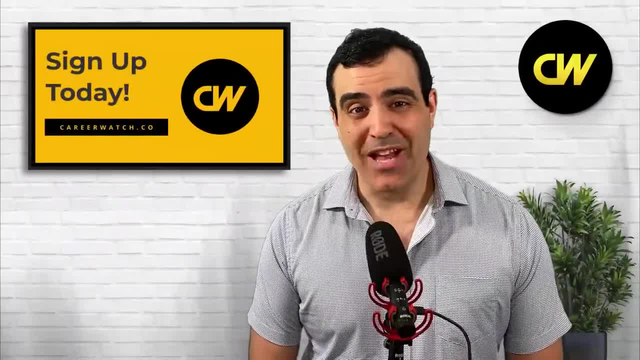 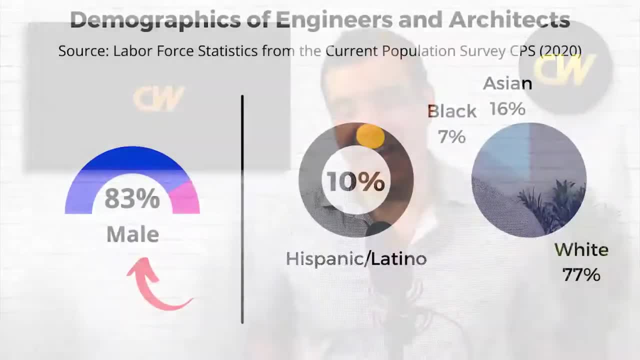 with urban and regional planners. Like every single other engineering discipline, environmental engineering is pretty male-dominated. It isn't as male-dominated as some of the other disciplines. About 83% of environmental engineers identify as male. 10% report they are Hispanic-Latino. 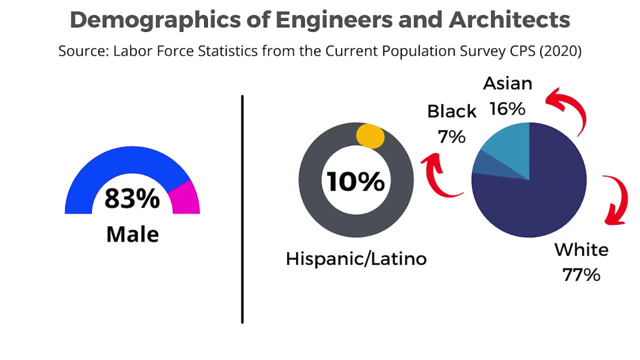 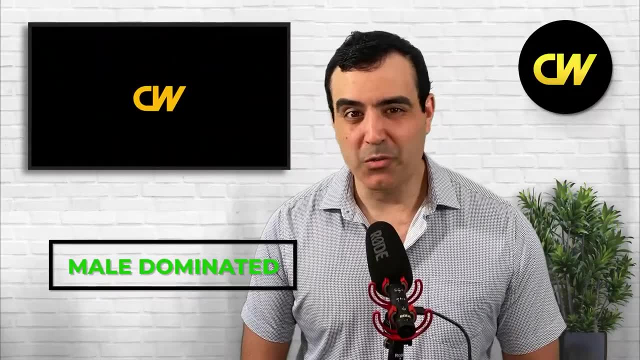 77% white, 16% Asian and 7%. This is definitely a pretty male-dominated occupation, although it's not as male-dominated as, say, electrical engineering, where about 93% of electrical engineers report that they are male. 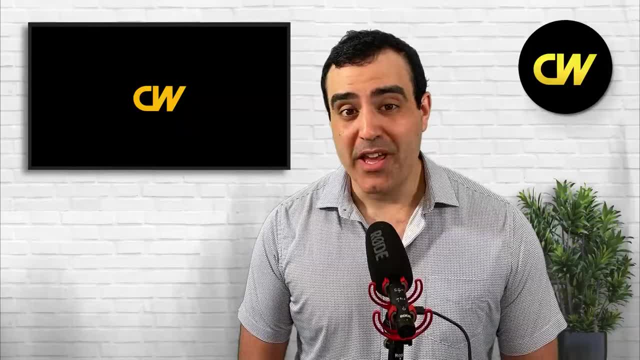 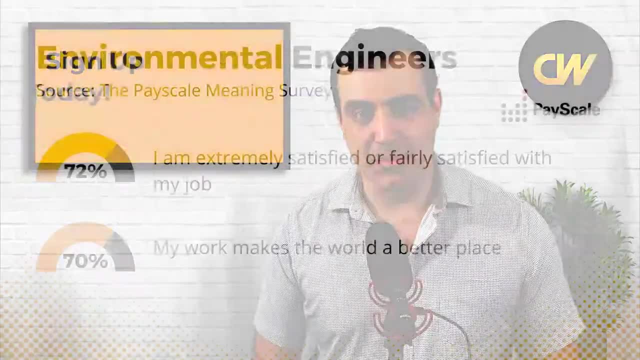 One advantage that environmental engineers have over other engineers is they tend to report higher job satisfaction and higher meaning in their work when you compare them to other engineering disciplines. This is from the Payscale Meaning Survey. About 72% of environmental engineers in the survey reported extreme satisfaction and about 72% of environmental engineers reported extreme satisfaction. 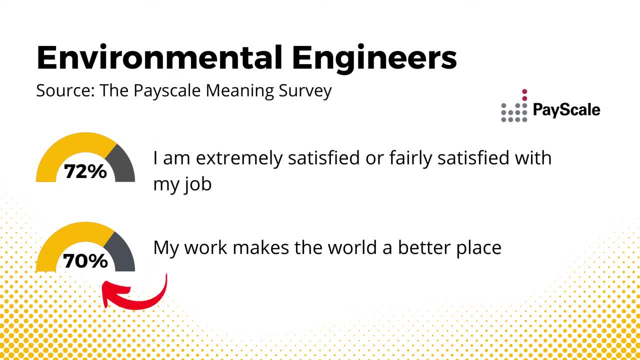 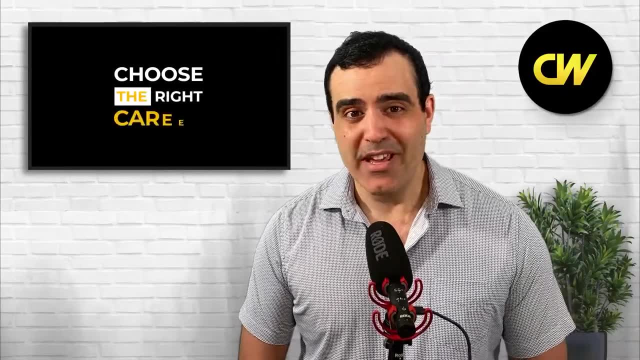 or fair satisfaction with their job, and 70% of environmental engineers report that their work makes the world a better place. Choosing a career that you find a lot of meaning in and that you're deeply satisfied with is one component of choosing a career. The thing is, many people choose the. 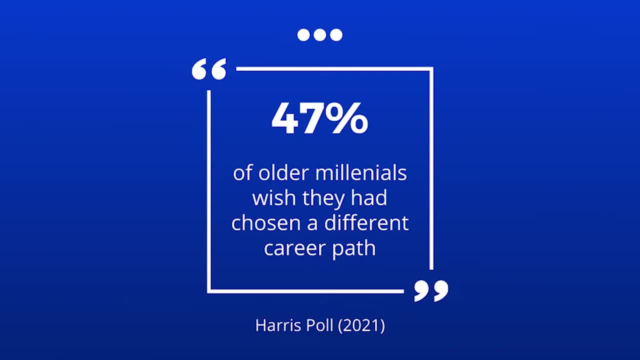 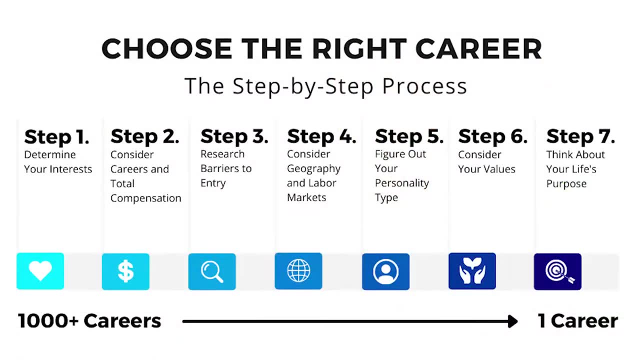 wrong career. In 2021, a Harris poll found that 47% of older millennials wished they had chosen a different career path. This is why we created a system for choosing a career called Choose the Right Career. This allows you to choose from 1,000 different occupations to that one right career. 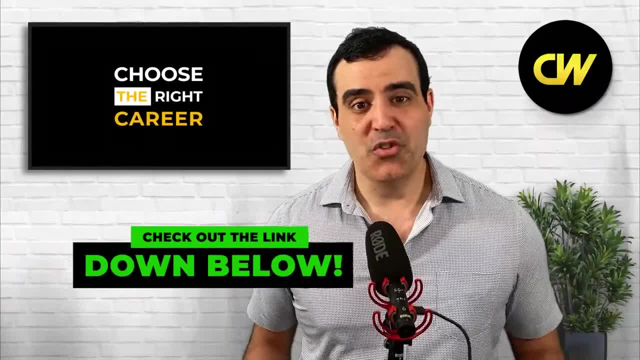 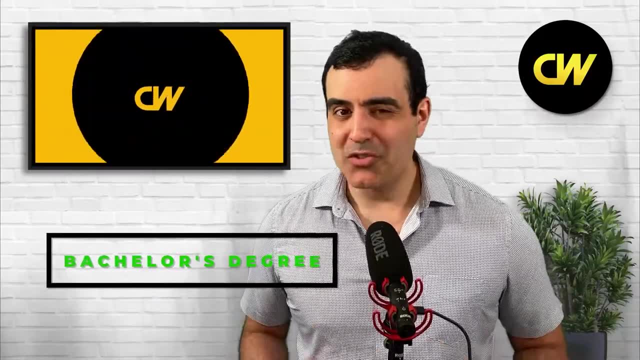 for you. Check out the link below. One advantage of choosing engineering over other fields is the fact that most engineering jobs just require a bachelor's degree. But when you drill down and you look at the 16 different engineering fields that are typically surveyed from the US government, you notice that there are certain 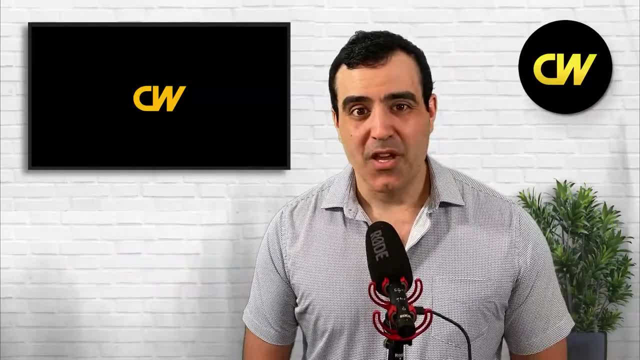 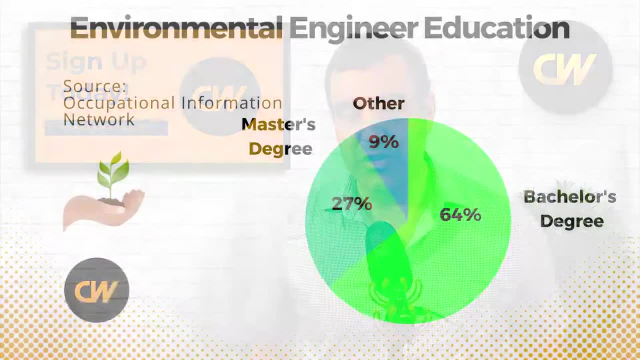 engineering fields that tend to require more education than others. For example, recently I did civil engineers and about 85% of civil engineers just need a bachelor's degree. For environmental engineers, about 64% of surveyed environmental engineers have a bachelor's degree. 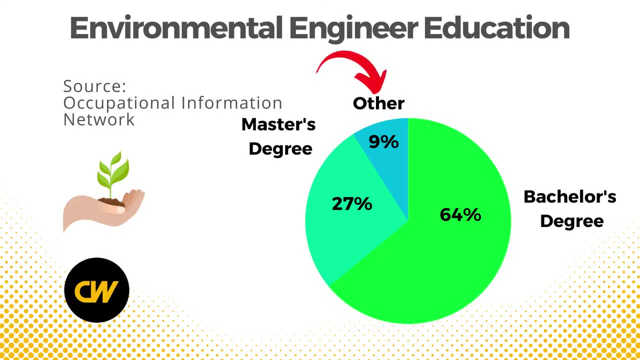 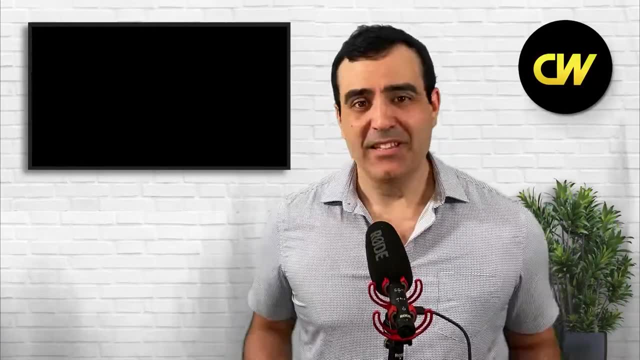 27% have a master's degree and 9% have other. So, compared to other engineering fields, environmental engineers tend to have more education than, say, civil engineers And, like civil engineers in other engineering fields, getting that professional engineering license. 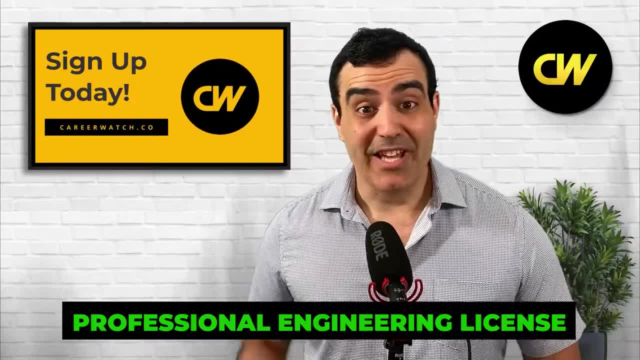 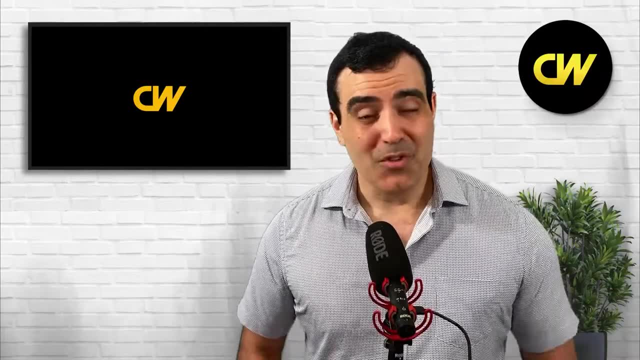 really helps you stand out from the crowd and get harder to get job opportunities. And what we're going to discover later is that there is demand for environmental engineers, but for some of the roles they're really actually pretty competitive. But first we're going to go into the 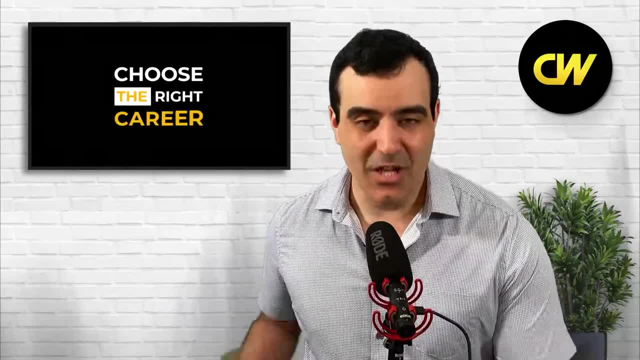 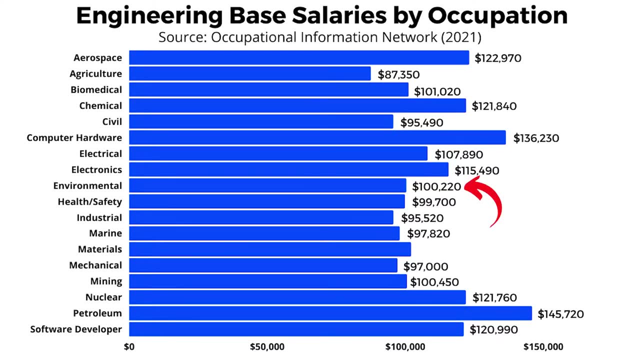 wages of environmental engineers, and we're going to compare them against the other engineering fields. In 2021, the average base salary for an environmental engineer was $100,220.. This means that, by average base salary, environmental engineering is the 10th most. 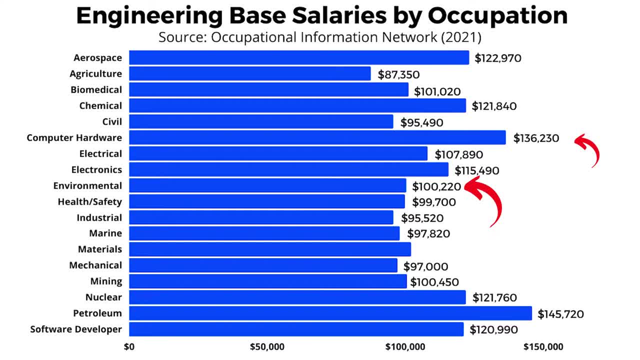 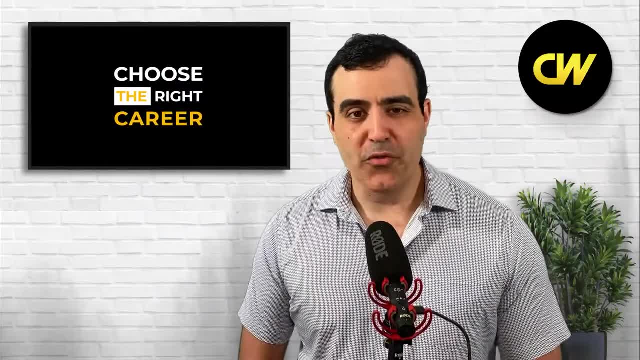 lucrative engineering field. It is beat out by fields such as computer hardware engineers, petroleum engineers, nuclear engineers and aerospace engineers, And environmental engineers have seen moderate wage growth over the years. In 2016,, the average base salary was $88,000. 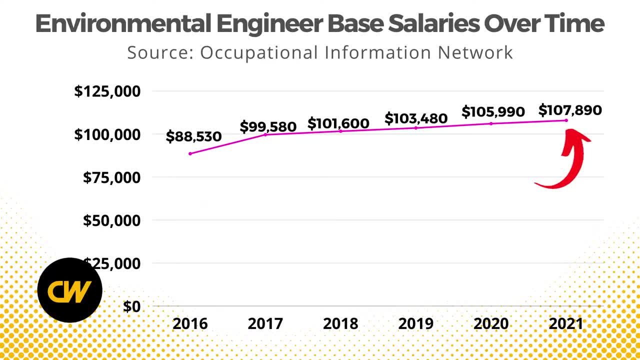 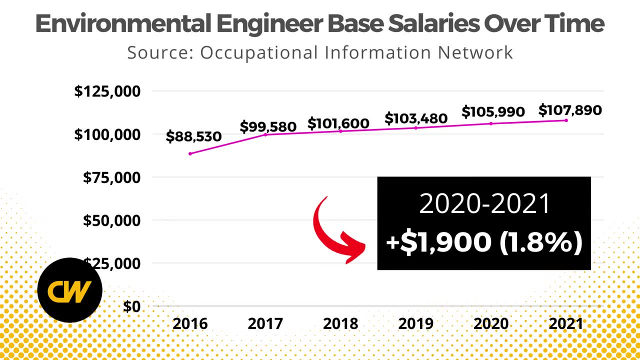 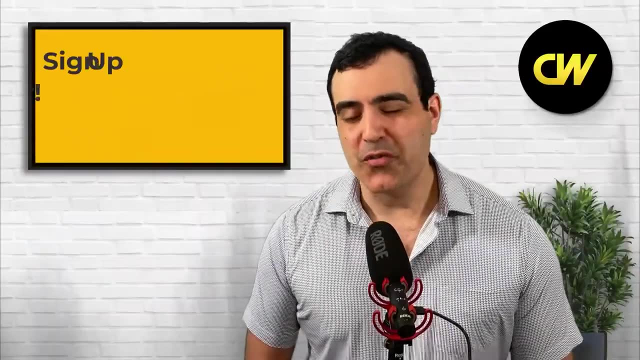 This average base salary rose to $107,890.. So between 2020 and 2021, there was about a $1,900 increase in wages for environmental engineers across the board, which comes out to a 1.8% wage growth. There's definitely some other engineering fields, such as aerospace engineering. 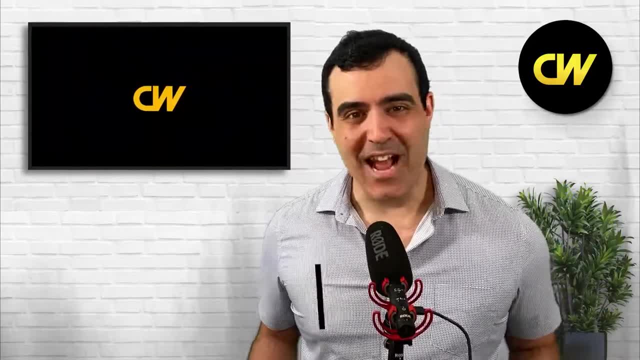 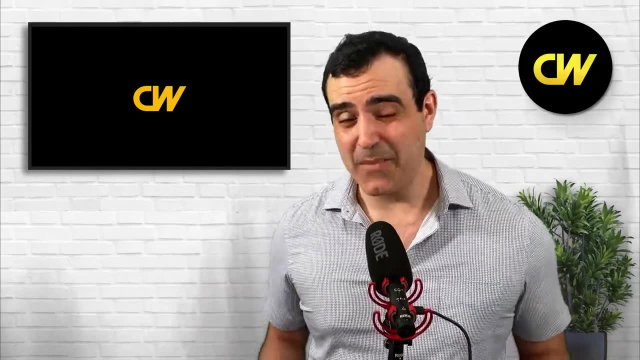 that are seeing faster wage growth than this. But keep in mind this is average base salary. There's actually certain metro areas that tend to pay environmental engineers a lot more than this. In fact, the highest paying salary for an environmental engineer is $1,800.. So that's. metro area for environmental engineers in 2021 is the Houston Texas metro area. You would think it'd be one of the coastal cities, maybe Los Angeles, San Francisco, Washington DC, Boston or New York, But no, it's actually Houston Texas, probably because of the oil and gas industry. 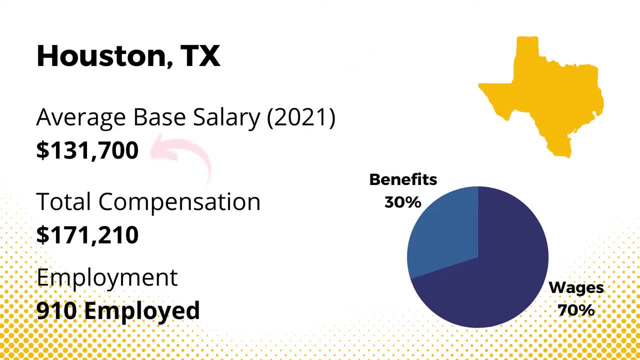 The average base salary for an environmental engineer in Houston Texas is $131,700.. Factor in benefits at 30%, Total compensation would be around $171,000 per year. There's about 970 employed environmental engineers in Houston Texas. The second highest paying metro is the San 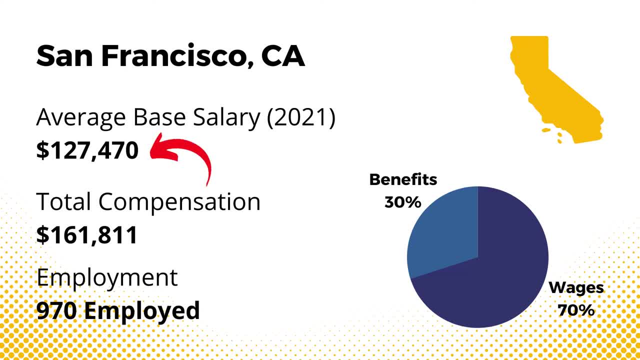 Francisco metro area, where the average base salary is around $127,000.. Considering 30% benefits, total compensation would be around $162,000.. And there's about 970 employed environmental engineers in San Francisco. Obviously, your money's going to go a lot. further in Houston, Texas, over San Francisco. San Francisco is extremely expensive. Next up, we have demand. What is the demand like right now for environmental engineers In 2022.? So we're actually going to look at Bureau of Labor Statistics data. 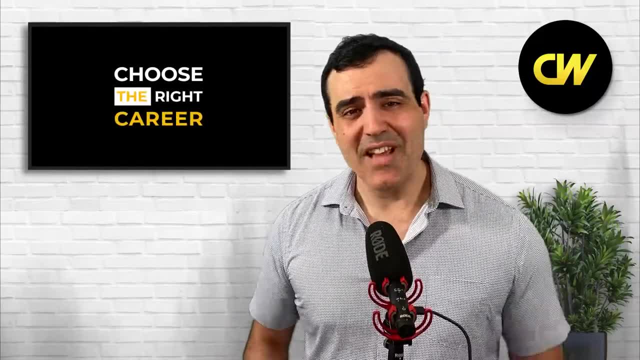 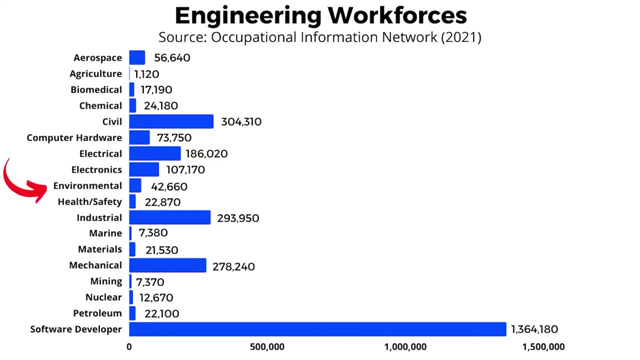 and we're also going to look at job postings. The first thing to understand is this is actually a pretty small workforce compared to the big three engineering fields. In 2021, the government recorded 42,660 employed environmental engineers in the US workforce. This is much smaller than 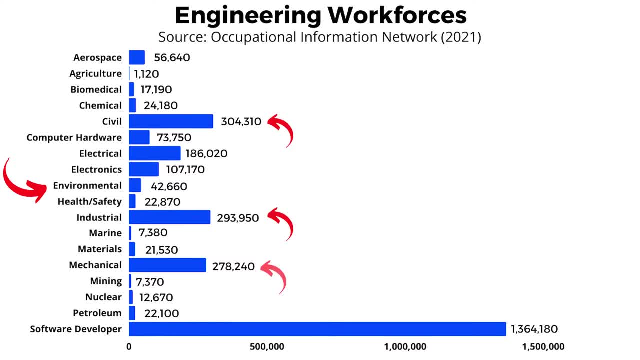 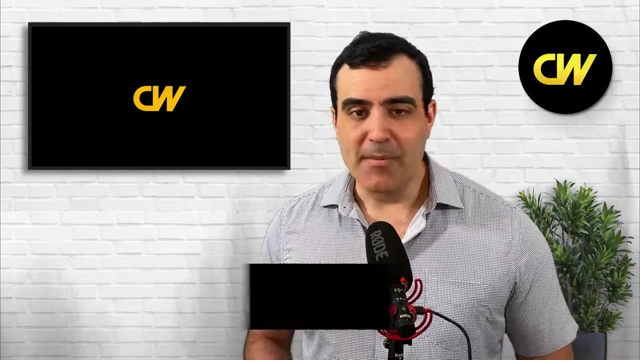 the number of employed civil engineers, industrial engineers and mechanical engineers, who all have around 300,000 people, And the environmental engineering workforce is significantly smaller than the number of employed software developers in the United States. This is a much smaller workforce than the big three engineering fields, meaning that job opportunities are going to be in. 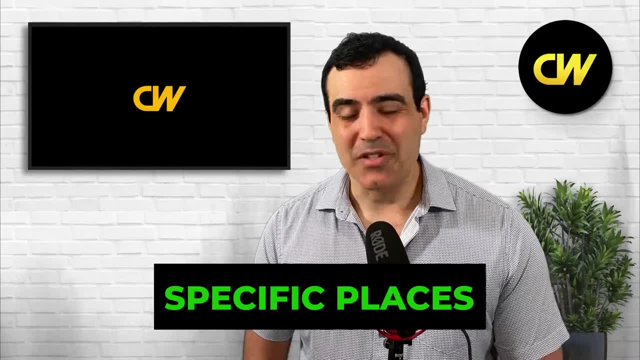 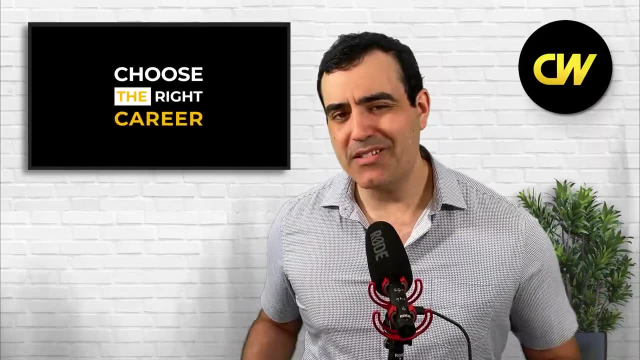 specific places and they're probably not going to be in certain towns and metro areas and even certain states across the United States. To make matters worse, the government is actually showing that there's actually been a decline in the number of employed environmental engineers since 2016.. 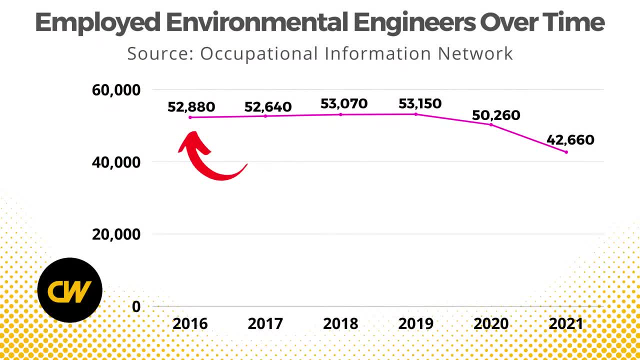 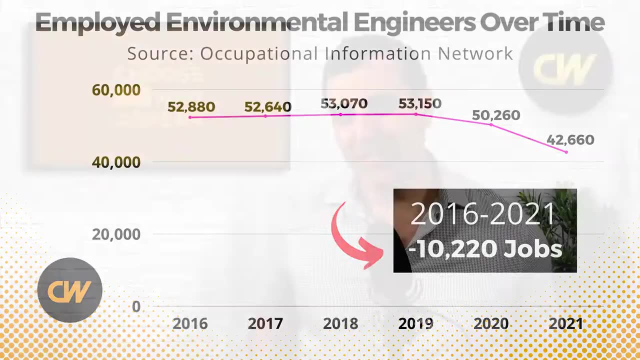 In 2016,, there was 52,880 employed environmental engineers. This dropped to 42,660 in 2021. So, between 2016 and 2021, the government recorded 10,220 less employed environmental engineers- Definitely not the best sign. This isn't the end of the world, because 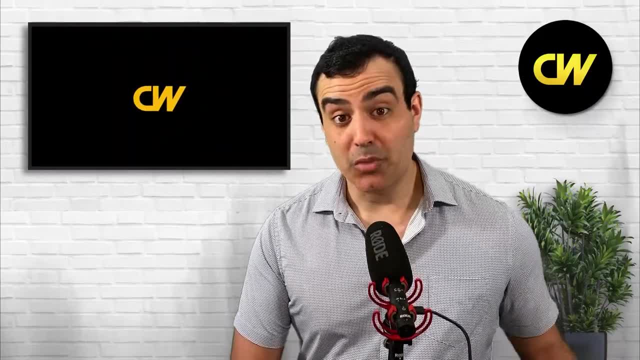 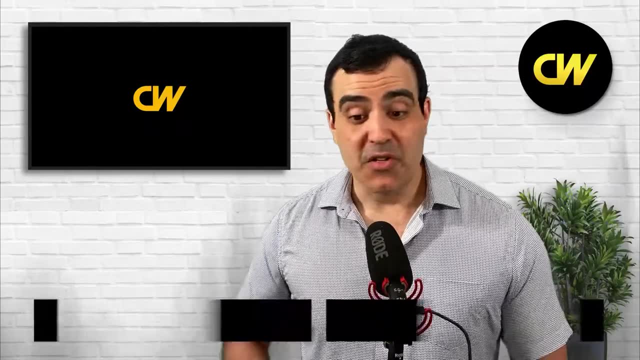 we're also going to look at job postings. but generally you want to see the number of employed people in your future career rising over time, not falling over time, Because if there's a fall in the number of employed, that means more and more people are going to be competing for those. 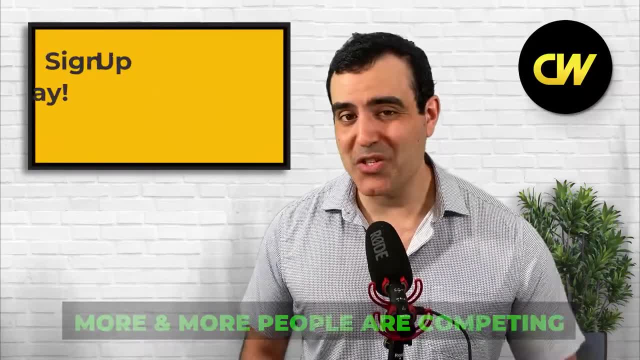 fewer number of employees. So that's a big thing. So that's a big thing. So that's a big thing. But fortunately the number of job postings right now for environmental engineers isn't kind of showing this. There's actually plenty of job postings for environmental engineers. 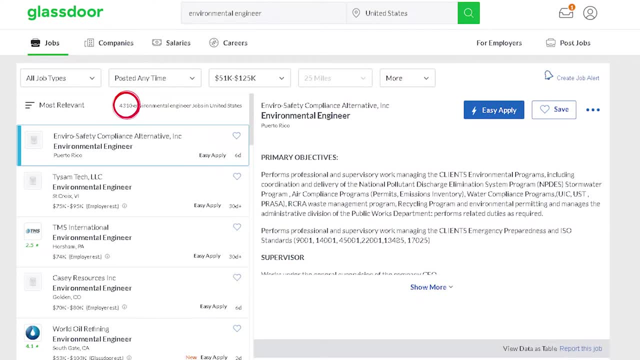 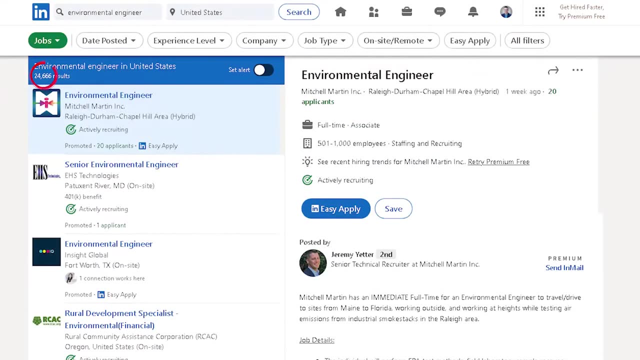 On Glassdoor when I searched for environmental engineer in the United States, there's about 4,320 job postings. On Indeedcom 8,714.. And on LinkedIn, around 25,000 job postings. So when you compare the number of job postings against the number of employed, it actually looks. 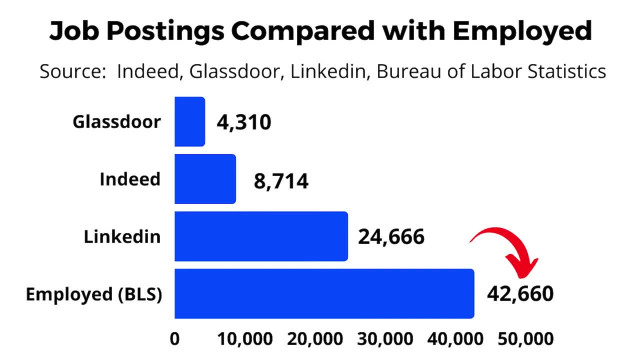 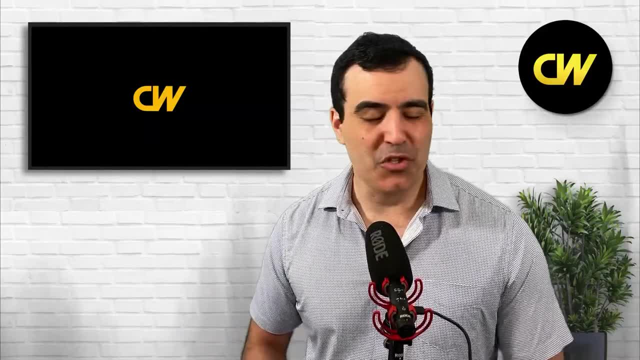 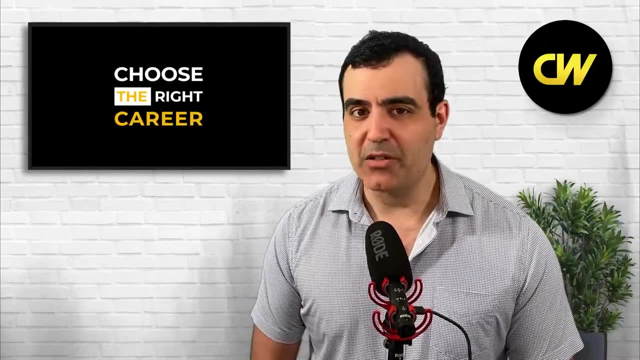 pretty good. It looks like there's plenty of demand for environmental engineers, Although LinkedIn there was a lot of software developers that came up that aren't environmental engineers- probably something to do with the algorithm on LinkedIn when you're searching for jobs. But even given that it really does look like there's plenty of demand for environmental 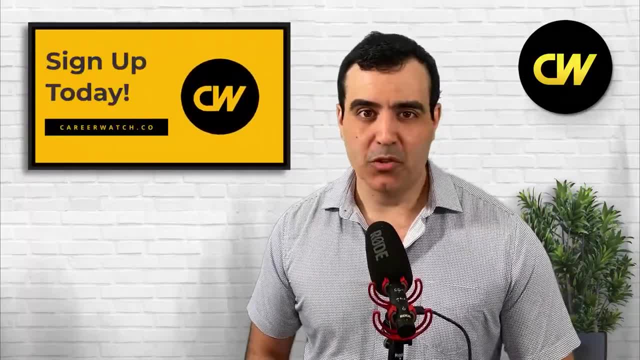 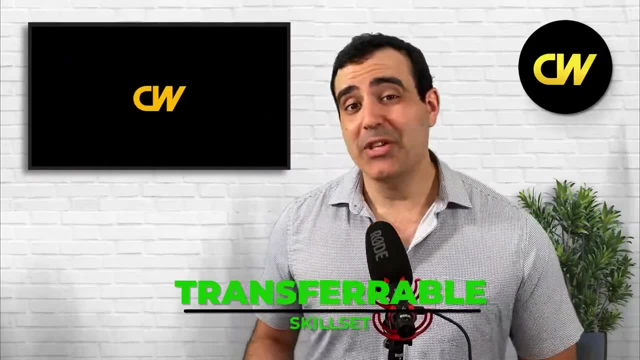 engineers And as an environmental engineer, if you go down this particular road, you're building a pretty transferable skillset that you can actually use in other engineering fields as well. Finally, we get into the personality of environmental engineers: Certain Myers-Briggs. 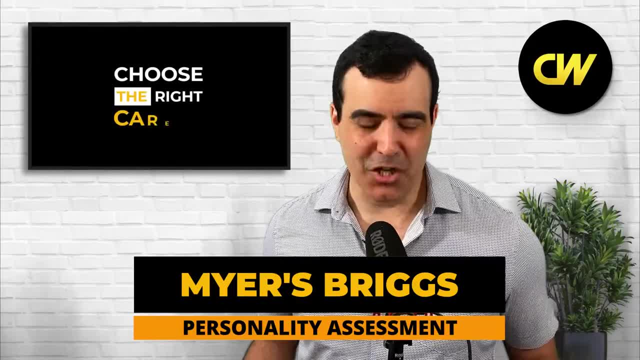 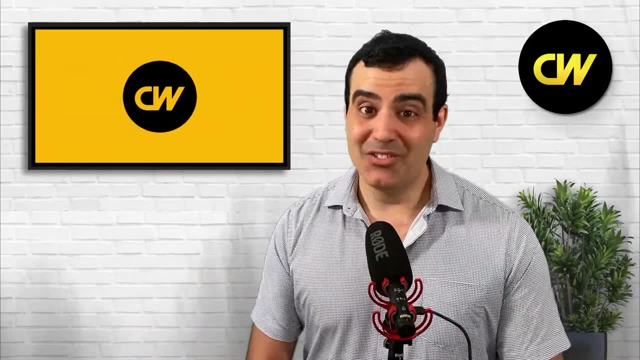 personality types are attracted to the job postings. So if you're looking for a job postings, this particular career slash occupation and others are not really that interested in it- And you're going. if you've watched any of my other engineering videos, you're seeing a certain theme. 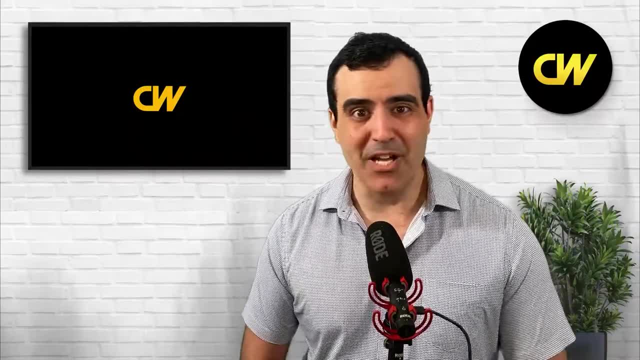 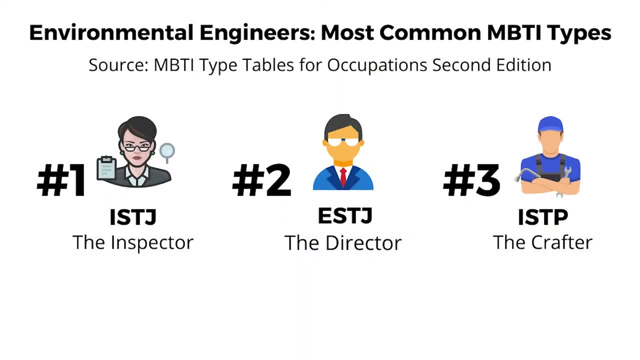 when it comes to the Myers-Briggs personality types, The same ones keep popping up because certain types are really attracted to engineering in general. According to the Myers-Briggs company, the most commonly found Myers-Briggs type in environmental engineering is the ISTJ. 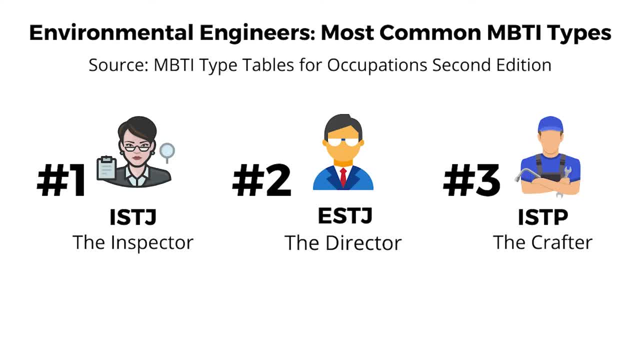 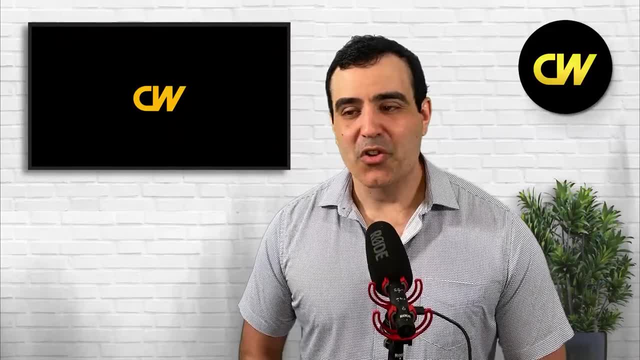 the inspector, followed by the ESTJ, the director, and number three is the ISTP, the crafter. If you watched any of my other videos, you'll see that there's a lot of different types of engineers. For content, you'll notice that the ISTJ and the ESTJ are two of the most commonly found types in